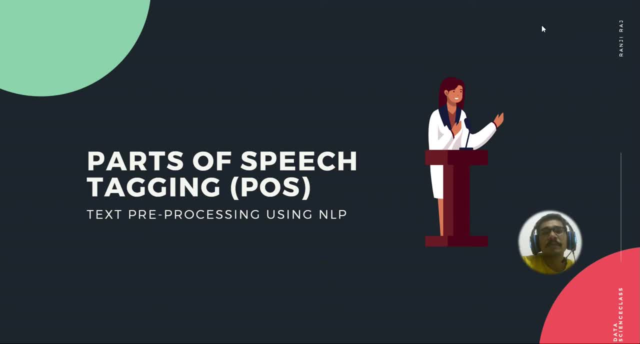 So those in a simple essence are called as parts of speech. So whenever you do NLP you have to deal with the English constructs also. So something or some part of the English language grammars are also involved whenever you deal with NLP projects or whenever you do any work with NLP. 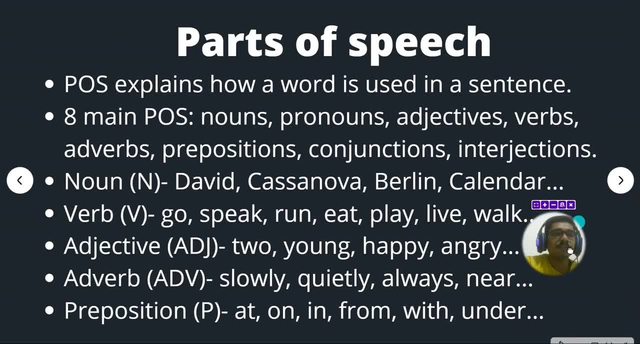 Okay, so let's jump on to the discussion. POS explains how a word is used in a sentence, So it gives its importance or significance. So basically, just talking about there are eight main POS, that is, nouns, pronouns, adjectives, verbs, adverbs, prepositions, conjunctions and interjections. 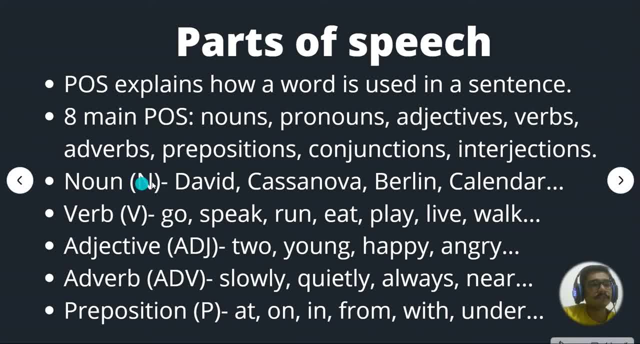 Okay, so a basic noun which is given as capital N. So name of any place, name of a person's, name of any object, any entity, everything which starts with capital letters, we have learned in that way, so those are categorized as nouns. so say, for example, david casanova, berlin calendar. so these 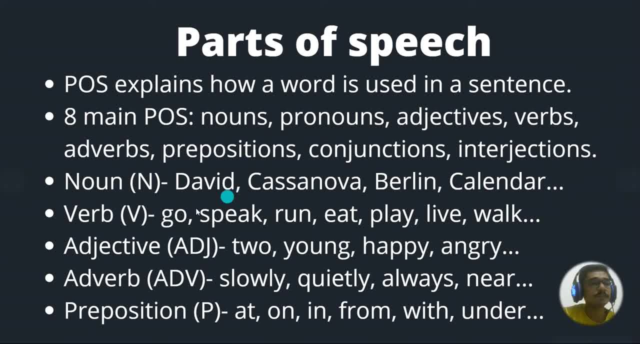 are given or classified as nouns. then we have verbs, so we have words like go, speak, run, eat, play, live, walk. those are basically verbs. i shouldn't be giving any further explanations on that. then we have adjectives. adjectives can include, i mean, if you ask me like how we can describe 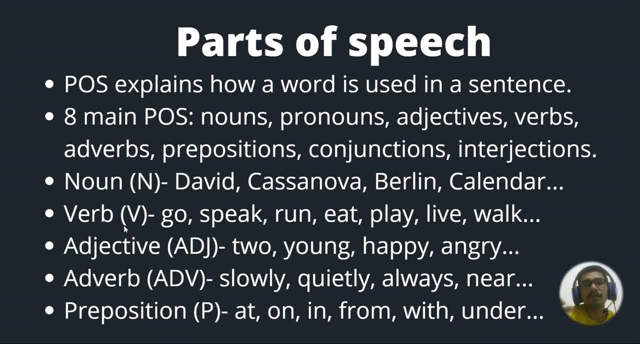 adjectives. so those are helping nouns. so for a noun it will be a word that is attached before that. so that will be basically you describing nouns. okay, so it can be also a number, like two, then young, happy, angry, like that. then we have adverbs so slowly, quietly, always near, like that. there are many in the 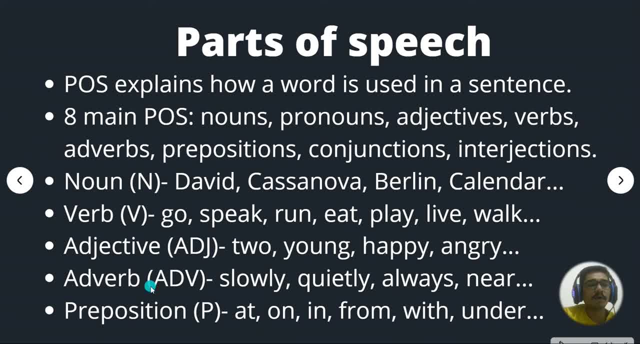 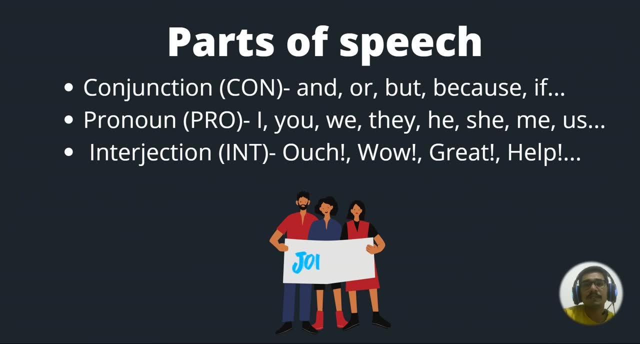 literature. then we have preposition at, on in from, with, under, beneath, above, like that. so those, everything comes under parts of speech. so there are a few more parts to it. so there are conjunctions which joins two words, that does, and, or, but, because if then we have pronounced i, you, be, they, he, she, me, us. okay, if you are addressing, 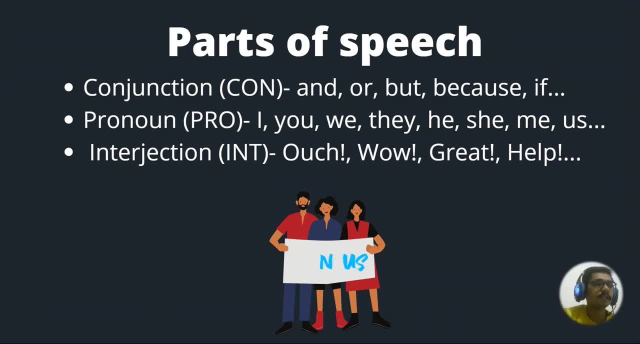 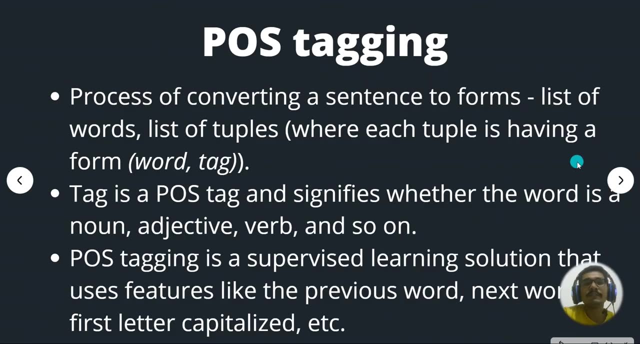 a person or a group of persons you basically use pronounced. then we have interjection, so its like with excremenation: Wow, great help like that. okay. So these are common parts of speech. Now let's move on to POS tagging- what this thing is basically. 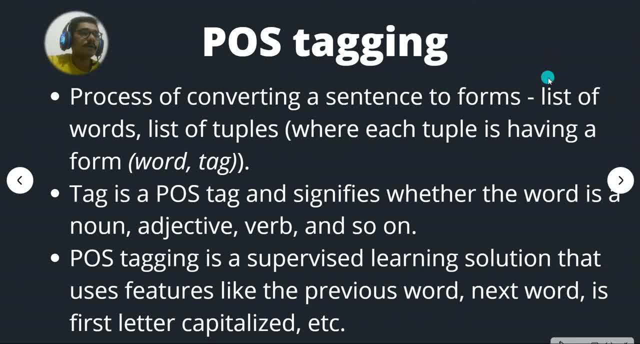 I'll just move to the upper left side. Okay, so POS tagging is nothing but the process of converting a sentence to form, basically, list of words, of tuples, So where you have each of the words and there will be some tags associated with that. okay, 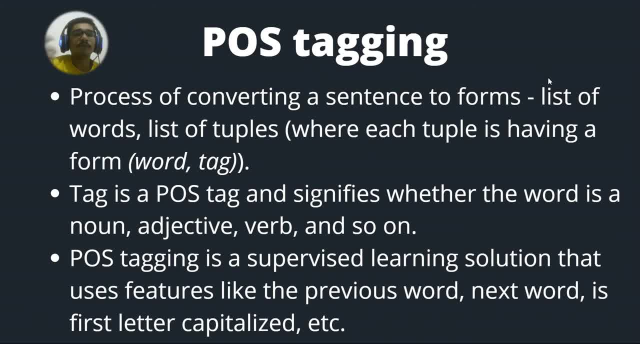 Okay, so each tuple will be having a form, So that will be a word and tag. So whatever words are there in that and before that we'll do the filtering for the stop words. So stop words are not included in POS, just the essential words and in which category they'll give or they fall under 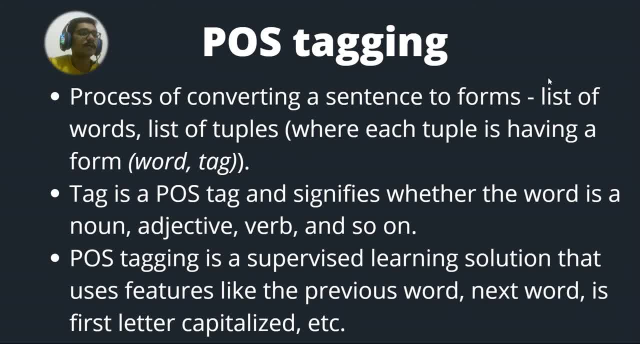 So for that we'll have a separate tag list that I'll be demonstrating you later. So tag is nothing but a part of speech tag and signifies whether the word is a noun, adjective, verb and so on, So that you can consider basically as a classification, how we can do that thing. 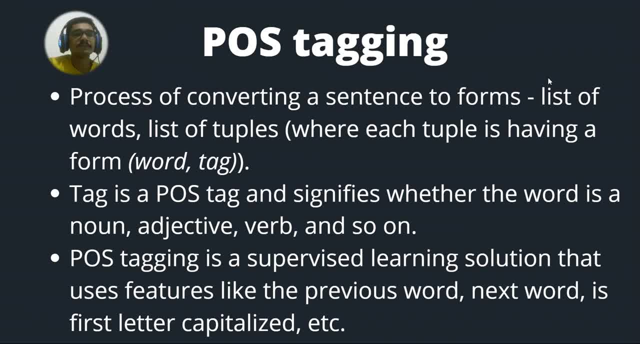 Okay so POS tagging is a supervised learning solution that uses features like the previous word, next word is the first letter capitalized, etc. and so on. Okay, so, since we have talked about like it uses supervised learning solution, there should be some supervised machine learning algorithm at the back end to do this activity. 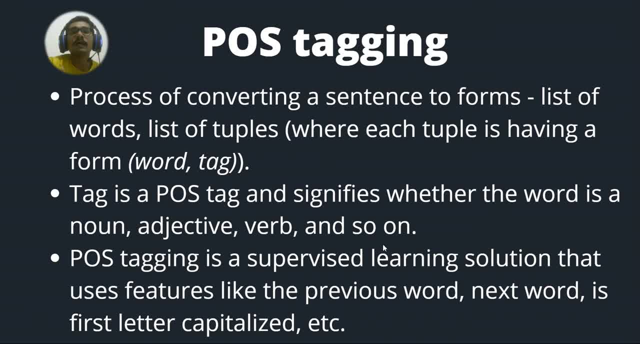 So to do that, we have a particular algorithm called as the average perceptron tagger. Okay, so this average perceptron tagger is the king behind all of this tagging process, So it does this activity. So before that, we talked about tags. 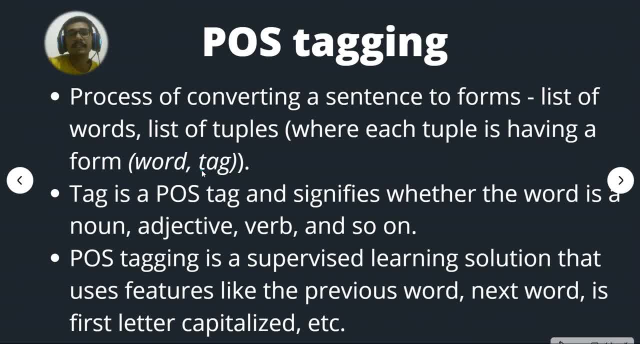 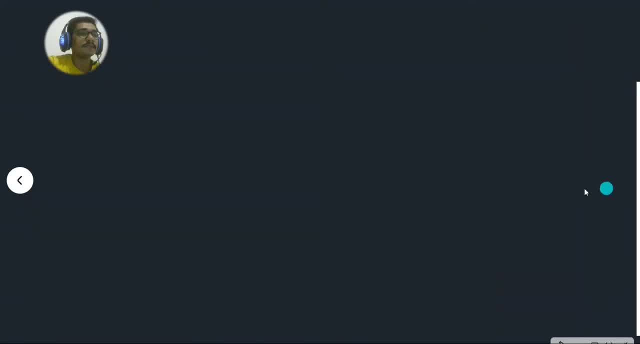 Tags is not the way which I have mentioned before. like N, A, D, J, There are a different set of tags under which these words are defined, So for that I'll just give an idea of this. That is, pen tree bank data set. 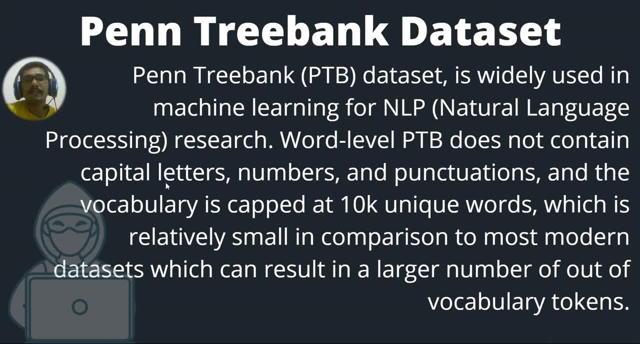 So this is actually a project that is pen tree bank. So these people, they did some activity and you can actually read. that is a PTP. data set is widely used in the ML literature for NLP research, So there they give word level PTP. 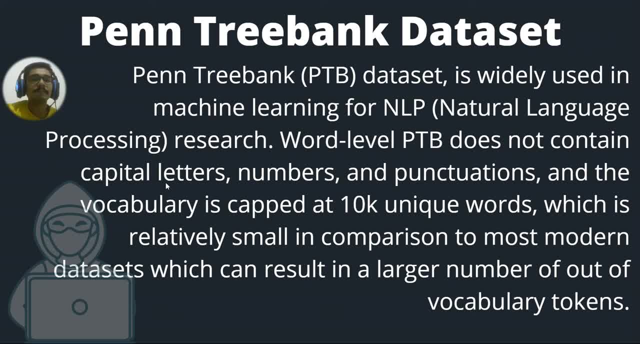 So any word level PTP does not contain capital letters, numbers and punctuations and the vocabulary vocabulary is capped at 10,000 unique words, which is relatively smaller in comparison to most of the modern data sets and can result in larger number out of vocabulary tokens. 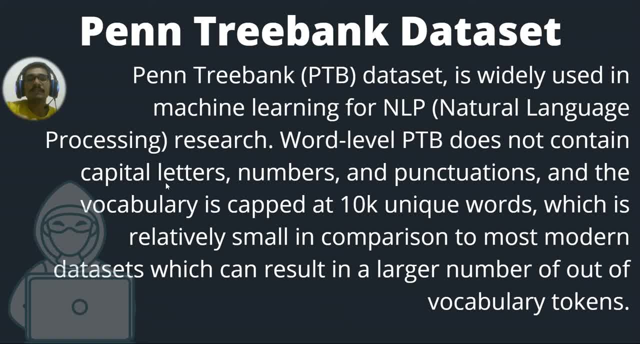 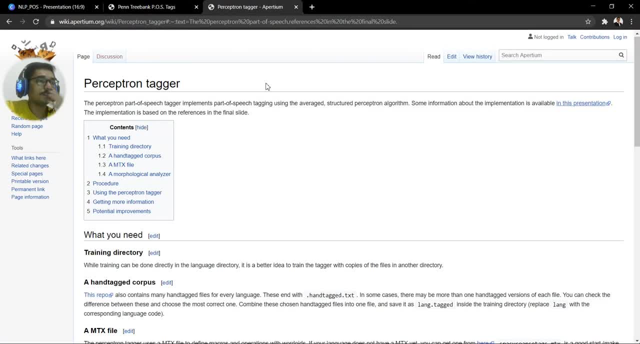 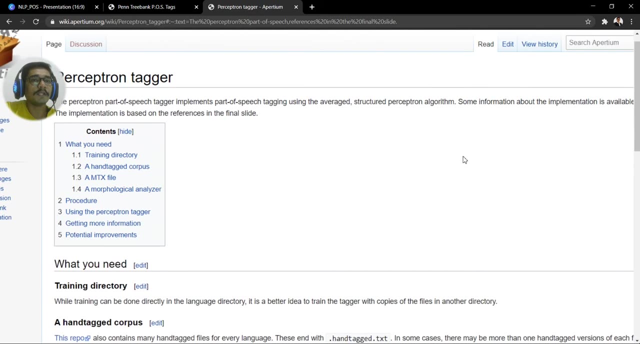 So let me first end this. Okay, So this was the perceptron tagger algorithm that I was talking about. So, as you can see, it implements POS tagging using the average structured perceptron algorithm. So you can read about this. 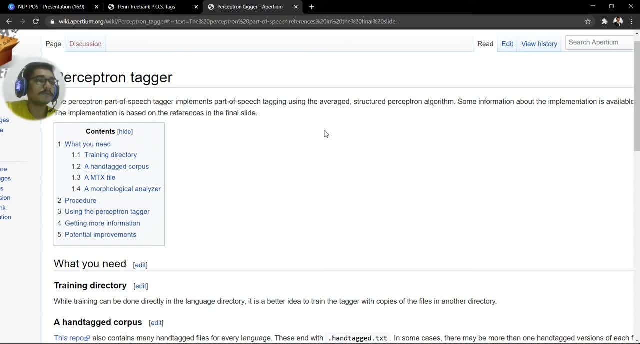 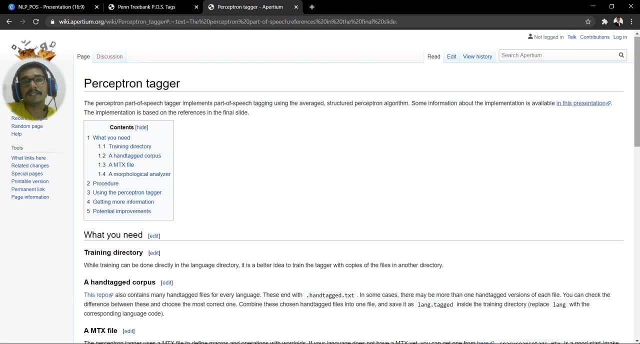 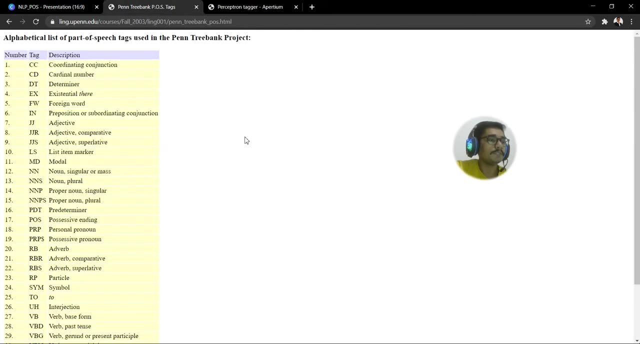 I'll just put the link in the description. Make sure you check this out. And also they have a presentation in which they talk about the implementation, how they did this perceptron, averaging for this different tags and talking about this tags. this is what we. 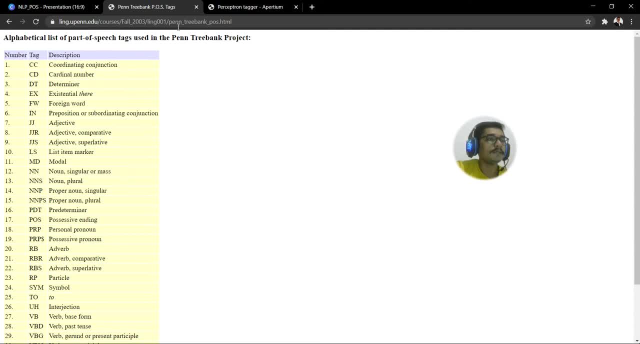 discuss. that is actually. this is a project which is done by the PTB project tree bank, so in 2003 they actually did this project and, based upon this project, they give their own specialized tags. so there are 36 unique different tags which are there, so for each of the tag you can find the description. so whenever 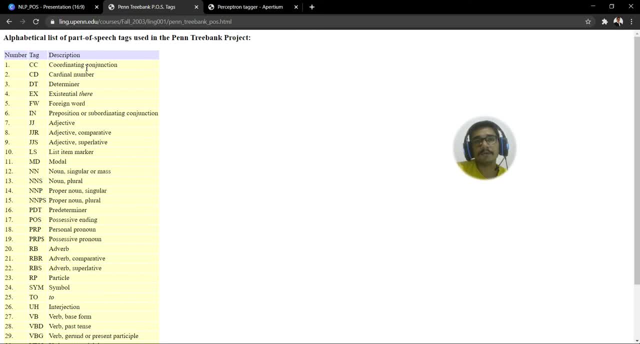 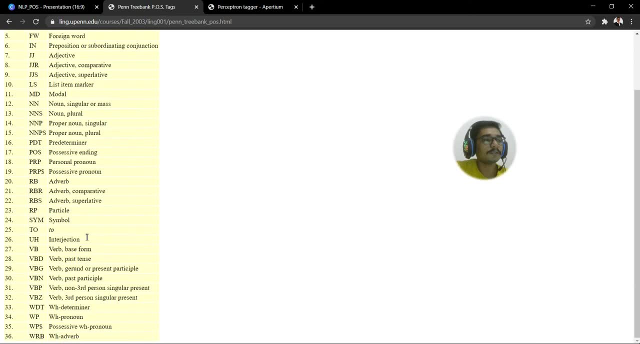 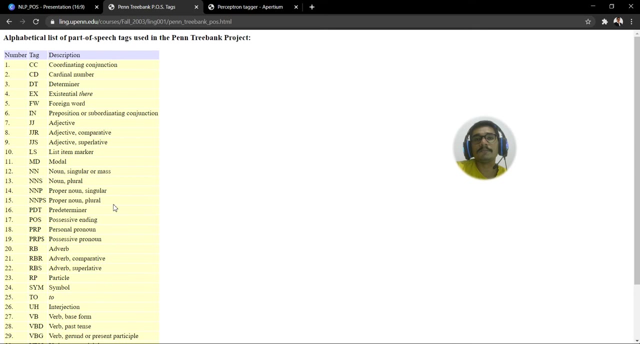 we do an NLP activity based upon this, POS tags, the tags which will be giving. we have to read out the meaning based upon this. okay, so there are 36 different categories or classifications for each of the words that we encounter, so let's quickly jump on to the python review of how this basically looks like. 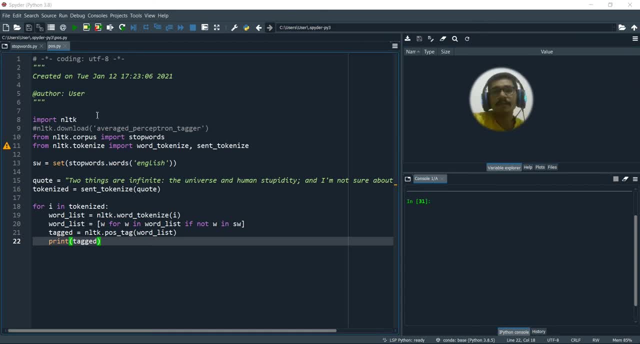 so this is my simple snippet to demonstrate what is a POS tagging. so first of all, I'll input NLTK natural language toolkit and you need this thing, that is, NLTK download. you have to download this for the first time. that is the average perceptron tagger, without which 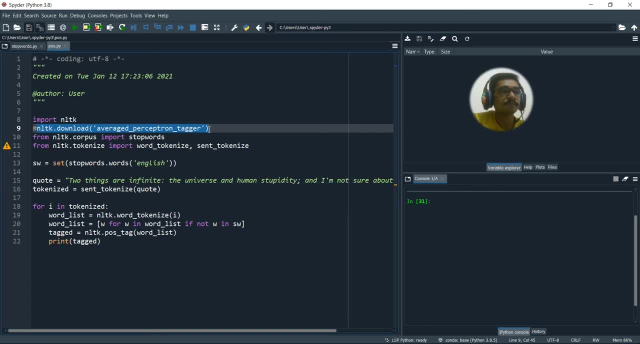 it cannot tag the words. it is as simple as that. so first you have to download this average perceptron tagger and then we'll be needing the help of stop words. okay, so from NLTK corpus, import stop words, then tokenize, word tokenize and sentence tokenization. 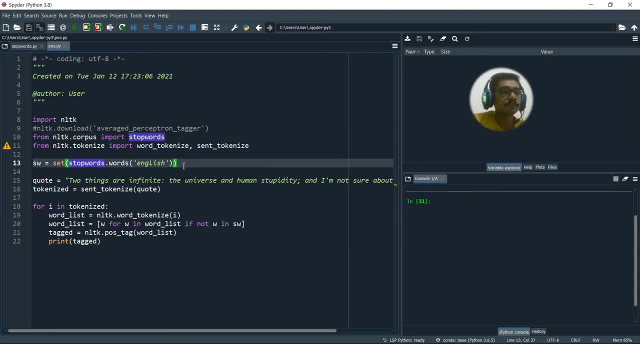 okay. so first we'll get the set of stop words which are there. so that's kept in an object: SW. so I'll take a famous quote from Albert Einstein: two things are infinite: the universe and human stupidity. and i'm not sure about the universe. so this is a quote. so this quote we have to tokenize first. so first I'll pass onto. 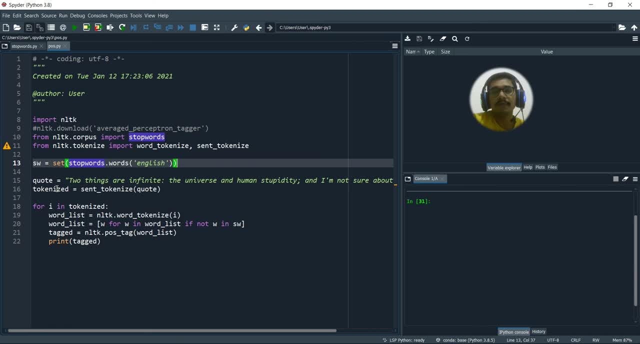 sentence tokenization, so you can use both ways: word tokenization, sentence tokenization. so first I'll tokenize this from sentence tokenization so I'll have the tokenized set here. so that will be a list, basically, and for each of the tokens which is present inside this I will pass into a word list. 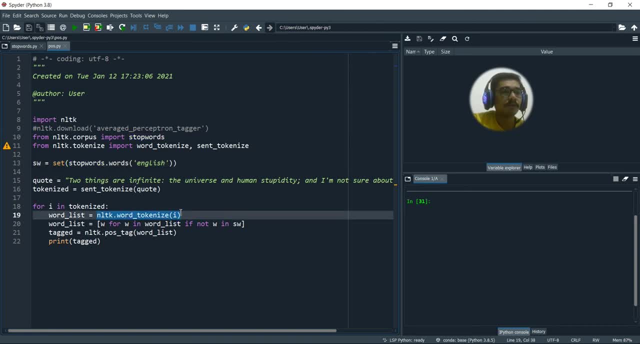 So that is nltkwordlist of word tokenized, and then what I will do is I will just refine this thing and I will just check if it's not content in these top words. So this is the filter that we append. So that is the same thing. we have seen before, this also. 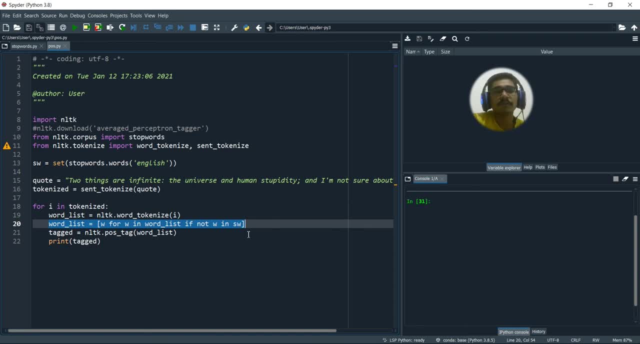 And for that words which are not there in the stock words, we will have a final set of word list which are just pertaining to that particular code or particular string. and for those particular tokens we will be attaching POS tags. So that is done by this particular function or method and we will just print the tagged. 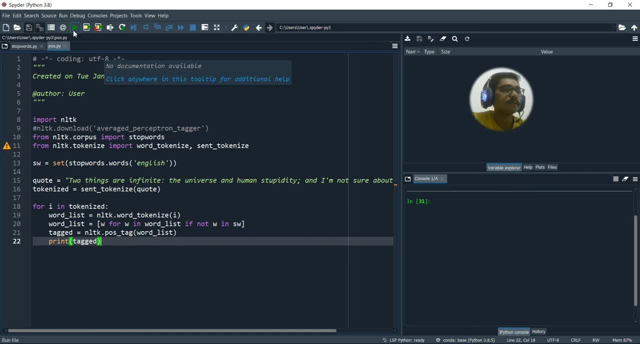 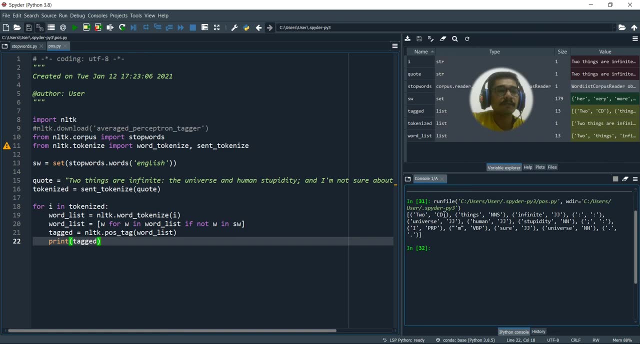 tuples, I mean the keywords, So that is clear. Then I will just run this. As you can see from this, tu was given a cd. So cd stands for cardinal number. So, as you can see, it identified tu as a number. 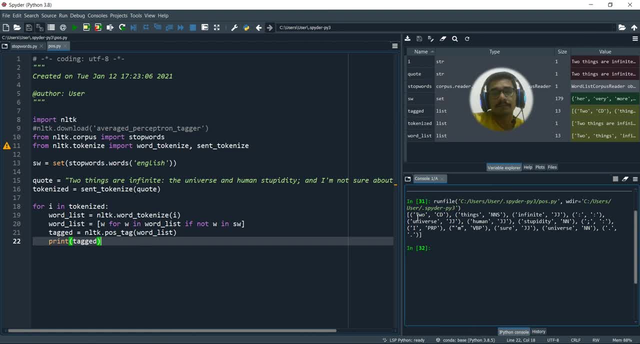 So now tu here is not in figures, but it is in words. okay, tw2.. So it is giving it as cd, cardinal number, Then things. So things were given as nns. So nns, It is nothing but noun and plural. 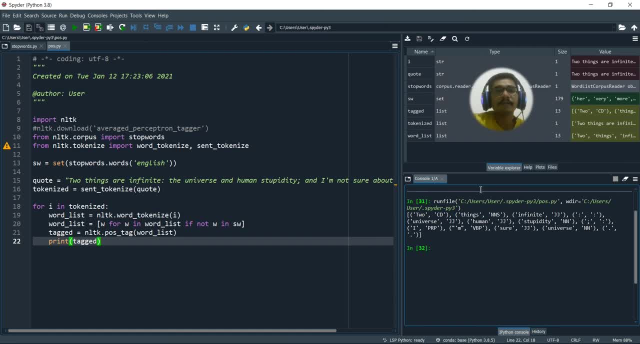 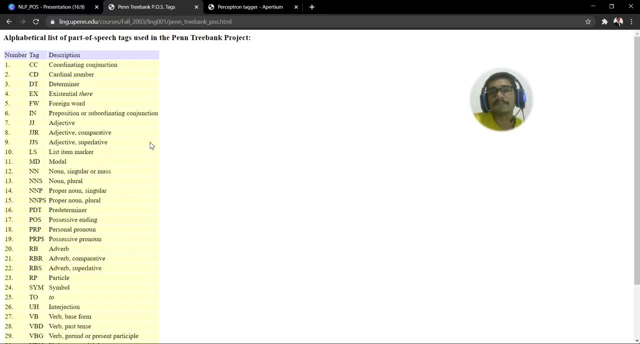 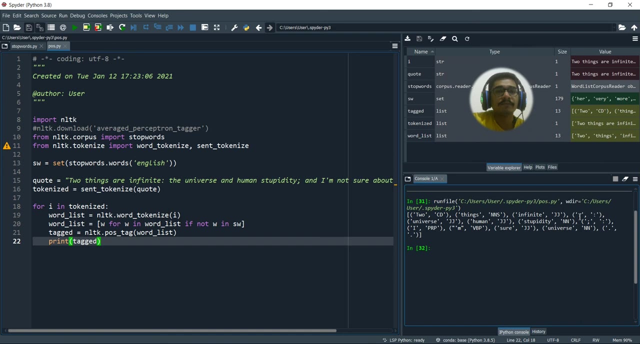 Yeah, it is right. Things. It is not singular object, but multiple objects. Then we have infinite. Infinite is given a tag as jj, which stands for adjective. Actually, it is a number. That is why it is given as adjective. Then we have some punctuation. 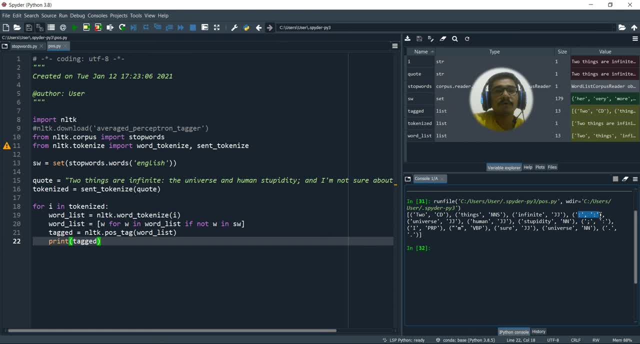 So punctuation, are classified as colon. So for colon and semicolon, both are given the same tag. Then again for universe, It is given as jj human. it is jj stupidity. it is nn, then i. that is for individual alphabet, That is prp. 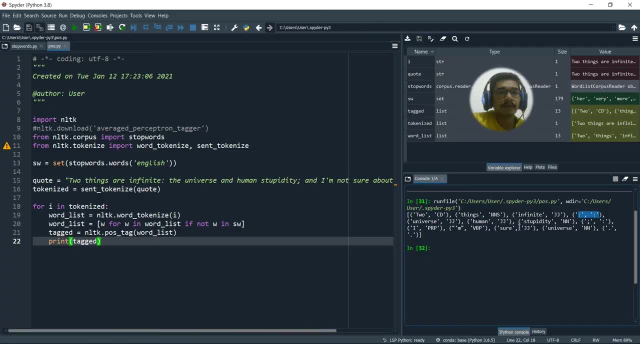 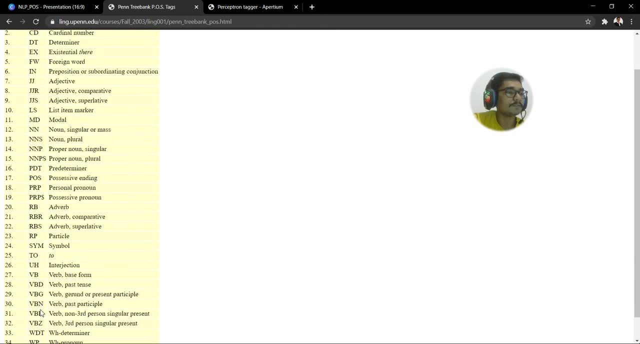 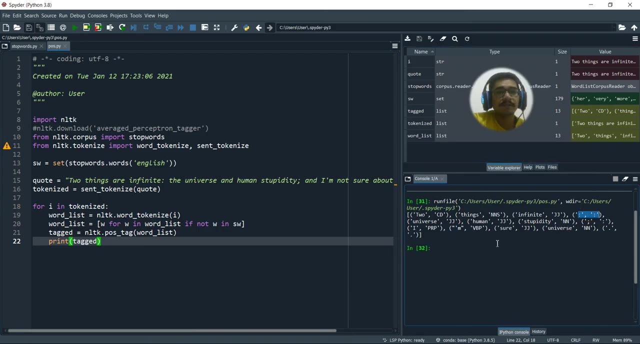 So prp stands for personal pronoun. okay, Then we have m. m stands for, or it is given as vvp, So vvp is for vvp, So it is given tags in this way. and sure is jj again, adjective universe nn. like that. 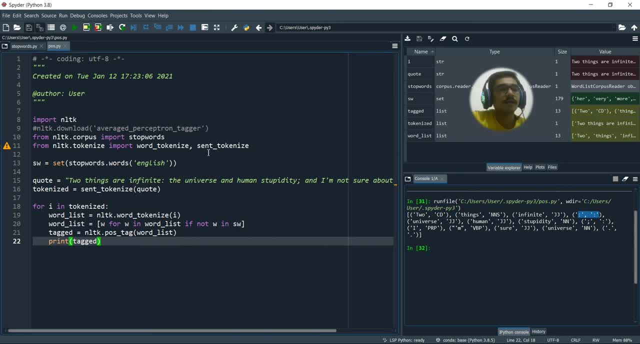 So this was a simple code that I have taken. but you can do an activity for very large chunk of text and you can basically do this. But this is done most of the time when you have a large corpus and just only for specific words you have to encode.